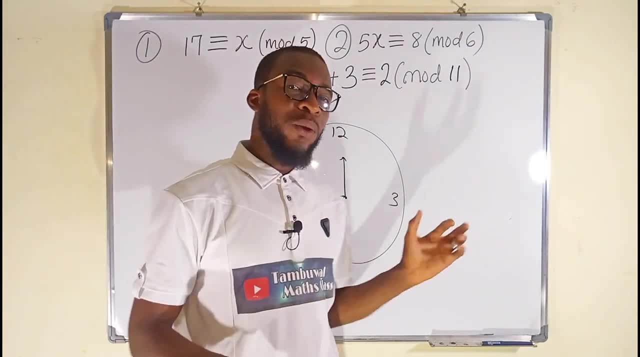 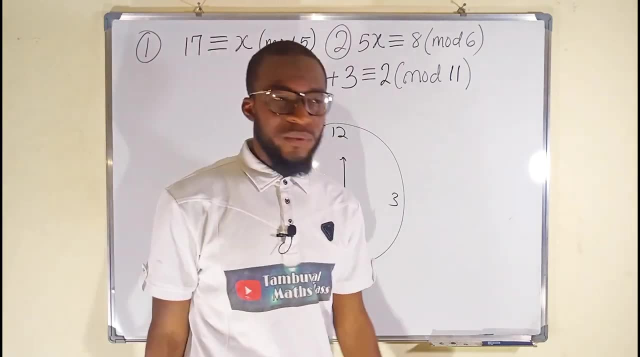 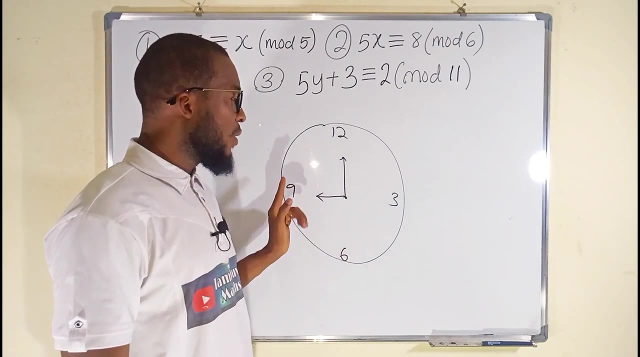 You should know that clock is either a mode 12 or 24.. It doesn't matter, because 24 is a multiple of 12.. So, now that we are at 9 o'clock, If I should add 6 hours from this 9, we are going to get to 3, because you know this is 10, this is 11. 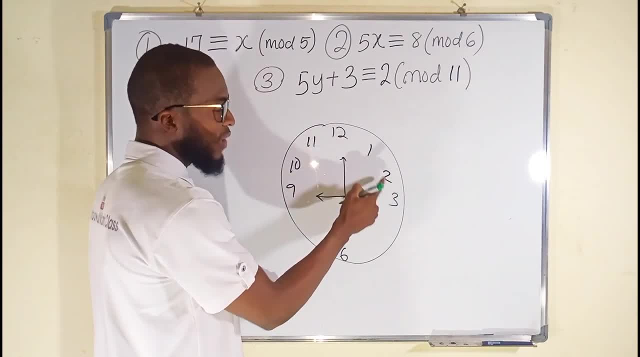 12.. So, now that we are at 9 o'clock- If I should add 6 hours from this 9, we are going to get to 3, because you know, this is 10, this is 11, this is one, this is two, so we have one, two, three, four, five, six. so, instead of 15, 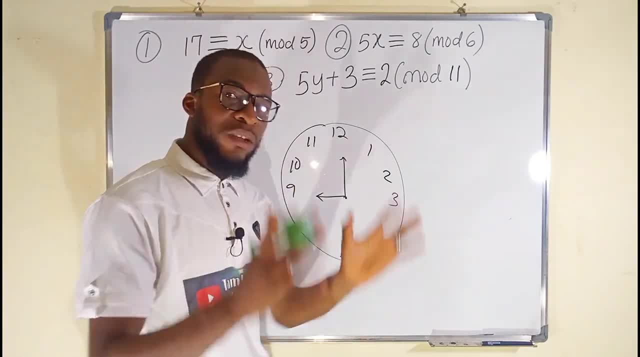 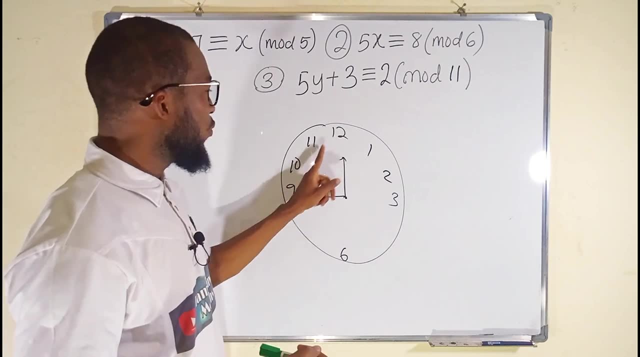 we have 30 because we are a mode 12. whenever you get to 12, you have to recount all over again from 0, 1, 2, 3, in that order. so we have 1, 2, 3. we have completed the bundle, which is 12. therefore, we have to complete that 6. 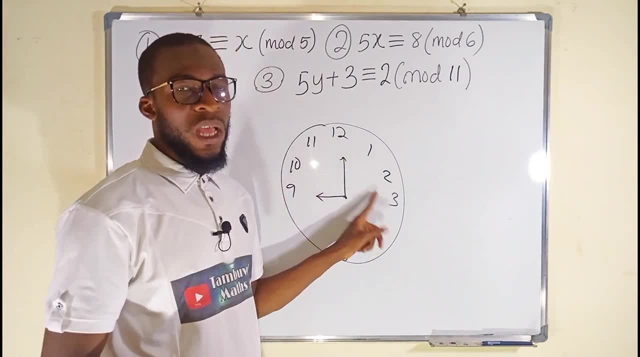 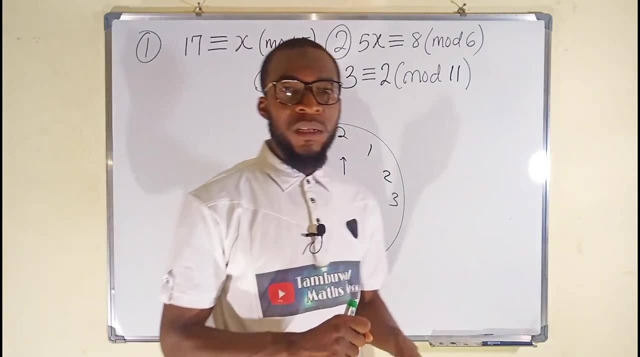 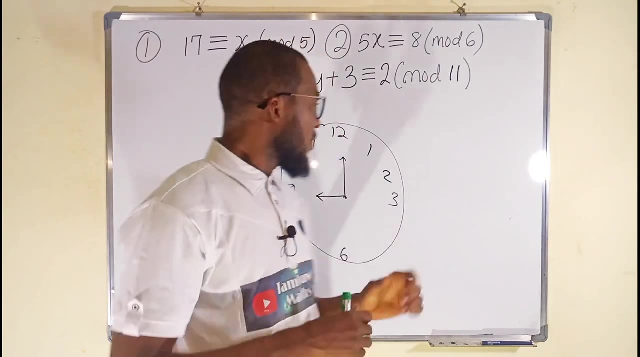 that we have started counting 1, 2, 3 and we get to this. and what about if we should add 12 for 9? if you should add 12, you will have to come back to that 9. this means that adding 12 to any number in much 12 is just like adding 0. what if? 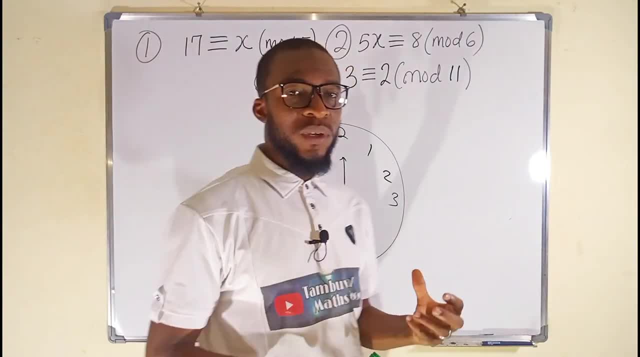 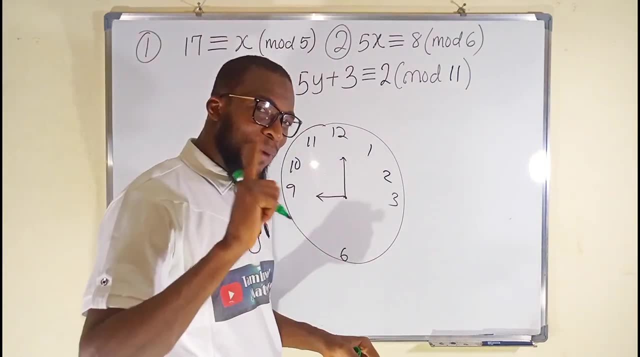 we should add 24. 24 is also a multiple of 12, so it's like we have not added anything. but what if we should add 25? remember, we are concerned with the remainder. so if you are 12, it will go back and come back to 9. 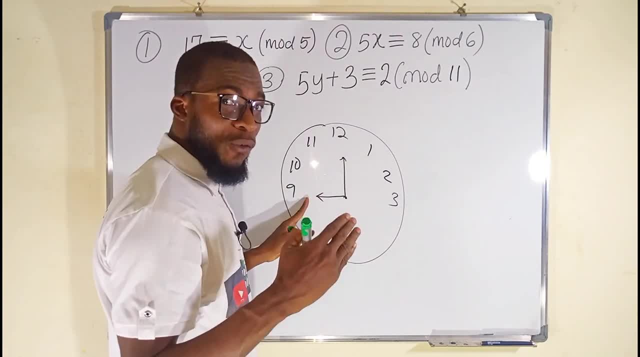 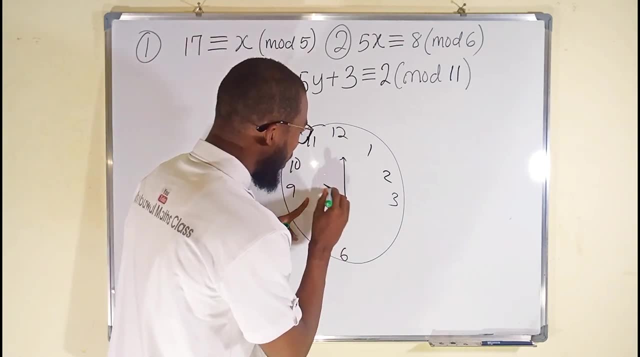 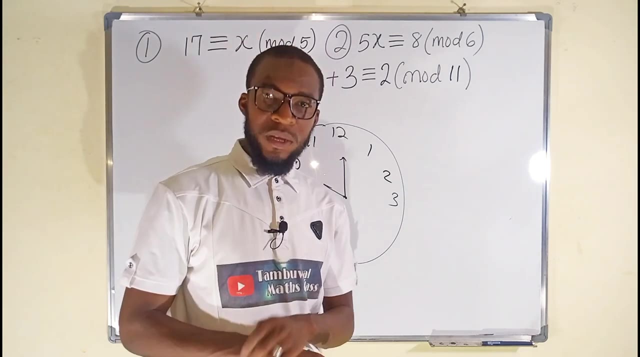 add another 12, it will go back and come back to 9, making 24. but we are talking about 25, we have one extra. so this, our hand, will look at 10 exactly. so if you should add 25, it will become 10 o'clock. this means that if you should divide, 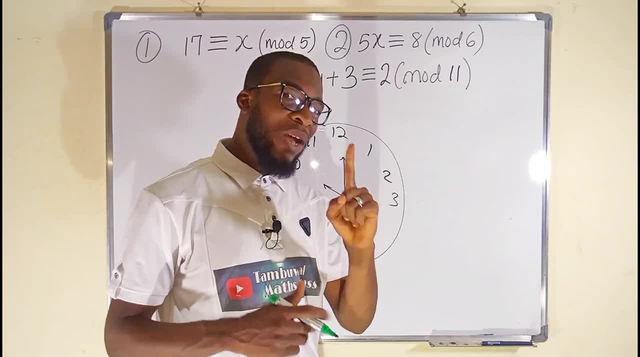 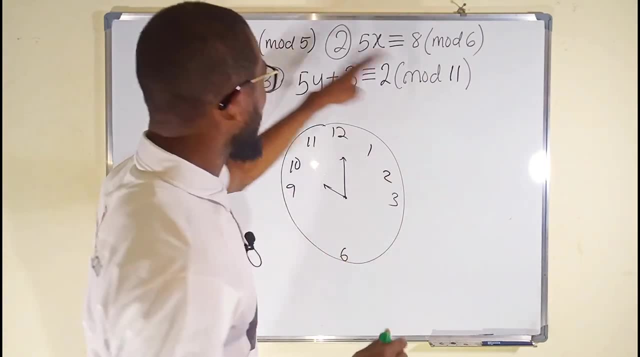 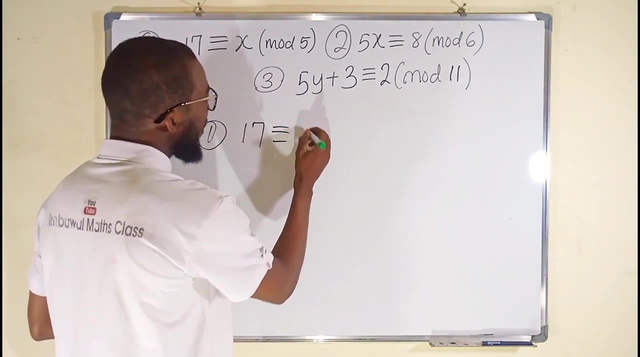 that 25 by 24, you have to get one with a remainder of one and you have to add that one extra which is going to make it 10. so now let us consider these three problems. the first one we have: the 17 is equivalent, a certain number, but a mod 5. what does this mean? it means that we are 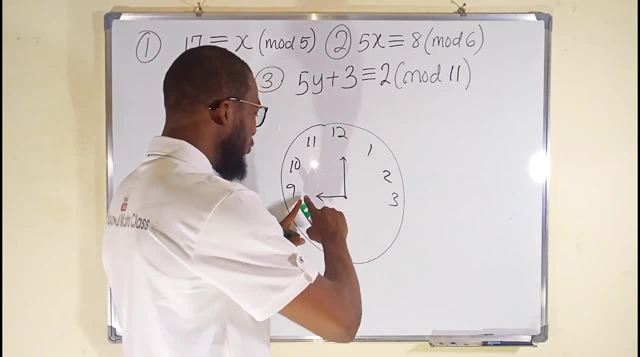 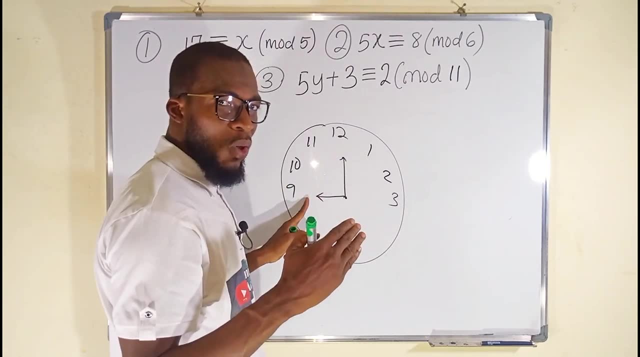 remember, we are concerned with the remainder. so if you are 12- 20, It will go back and come back to 9. add another 12.. It will go back and come back to 9, making 24, But we are talking about 25.. We have one extra, So this: 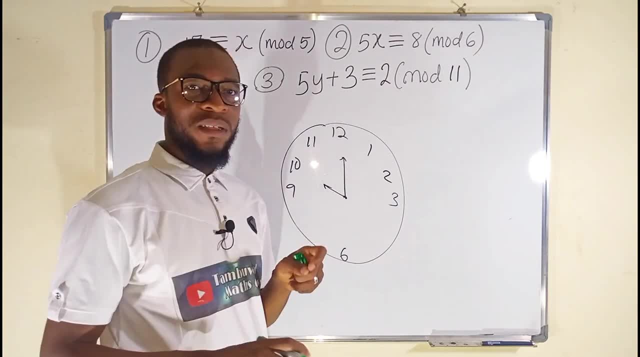 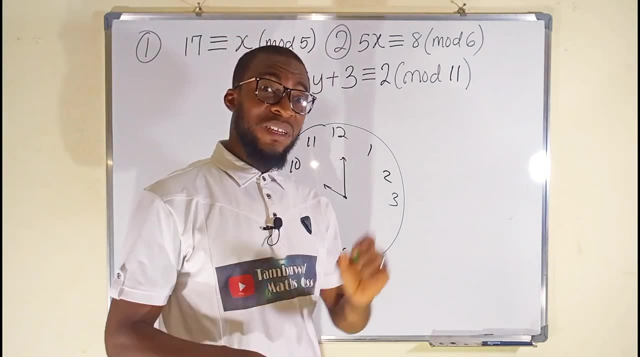 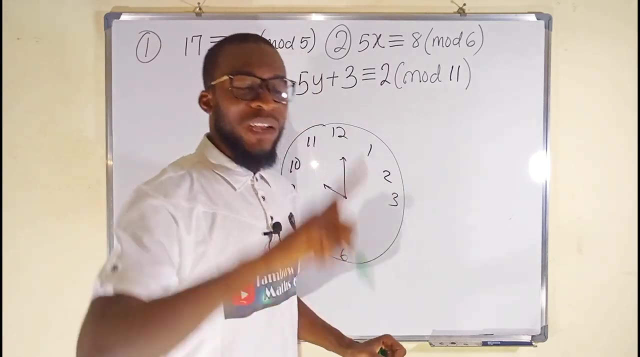 our hand will look at 10 exactly. So if you should add 25, it will become 10 o'clock. This means that if you should divide that 25 by 24, You have to get one with a remainder of one and you have to add that one extra. 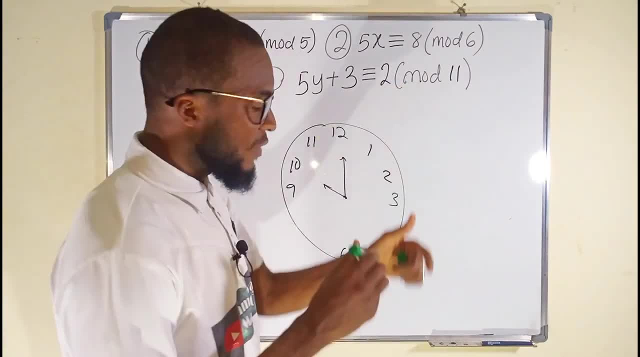 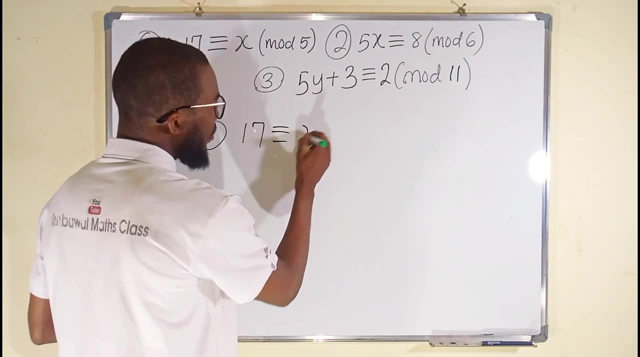 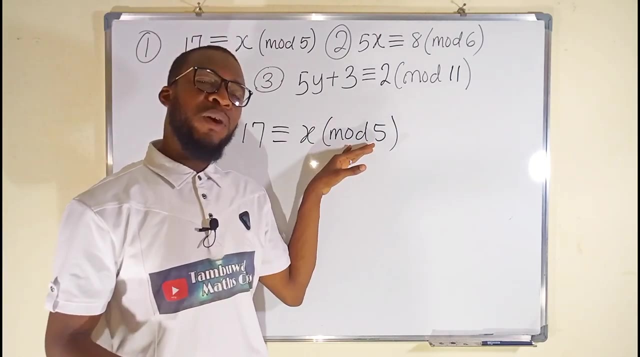 Which is going to make it 10.. So now let us consider these three problems. The first one we have: the 17 is equivalent a certain number, but a mod 5. what does this mean? It means that we are now talking about bundles of 5. 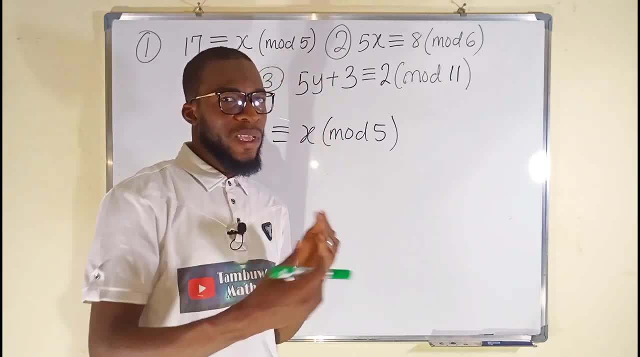 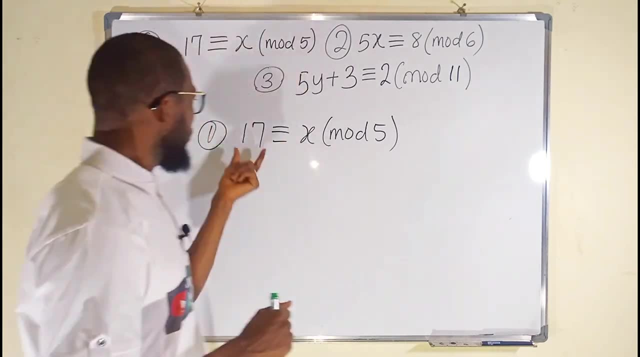 1, 2, 3, 4, 5. you recount all over again: 1, 2, 3. All the countings will be based on 5, which is a complete bundle, So 17. how many bundles of 5 are there in 17?? We have three groups. 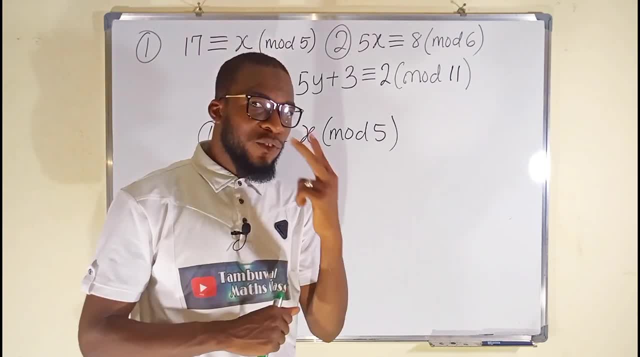 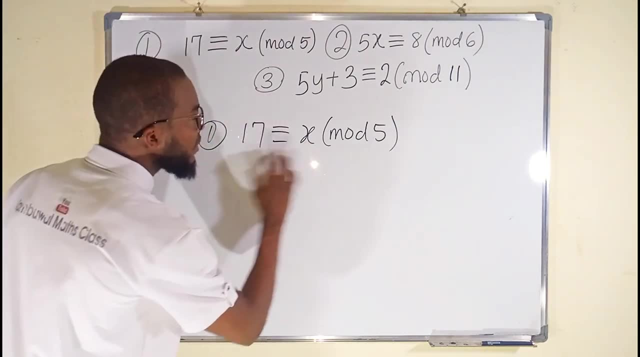 Well, let me say we have three bundles with a remainder of 2.. So this number right here is just our remainder. What does this mean? It means that if we should divide 17 by 5, What is going to be the remainder, and that remainder is going to be our solution. 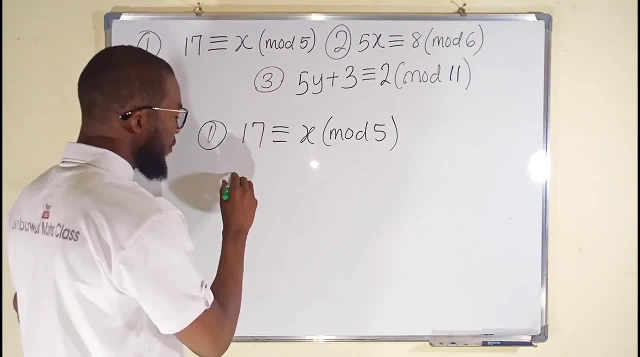 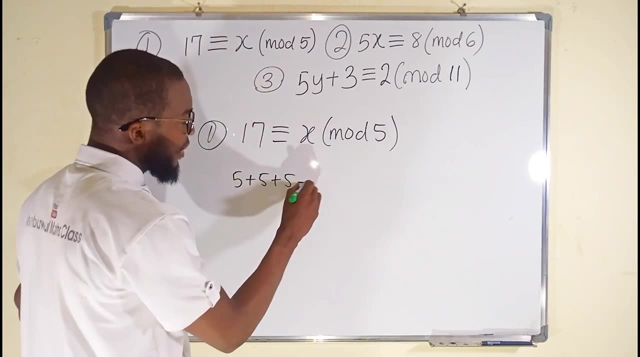 So this time around you can even do it practically. you say 5 plus 5 plus 5, since we are counting in bundles of 5. This is 15, then plus 2.. Can you see, this is complete bundle, where we have a remainder of 2 and 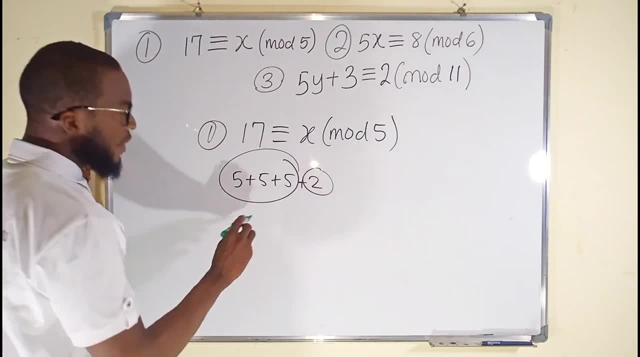 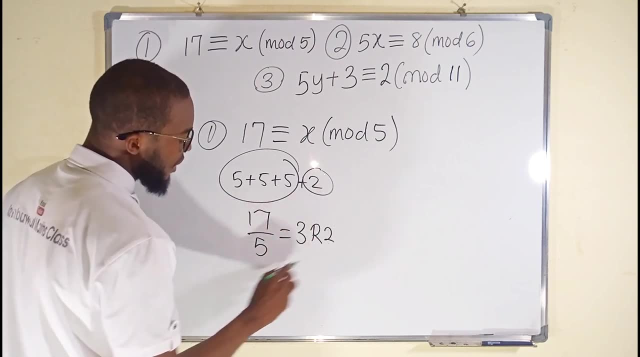 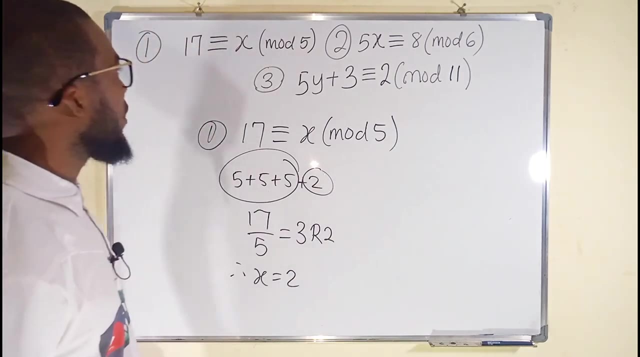 Therefore this X is equivalent to 2. another way you can do that is to say that this 17 Divided by 5 is equal to 30, which remainder of 2, and therefore X is equal to 2, But only in mod 5. Okay, second question: We have that 5x is equivalent to. 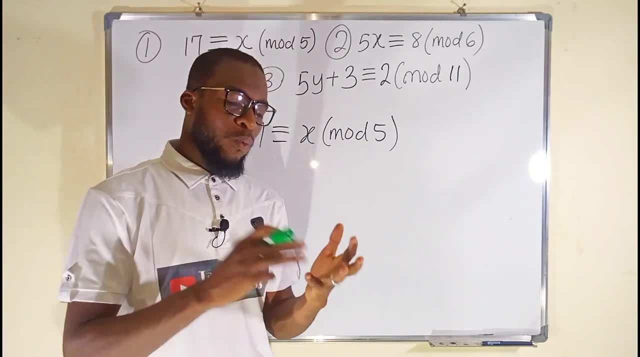 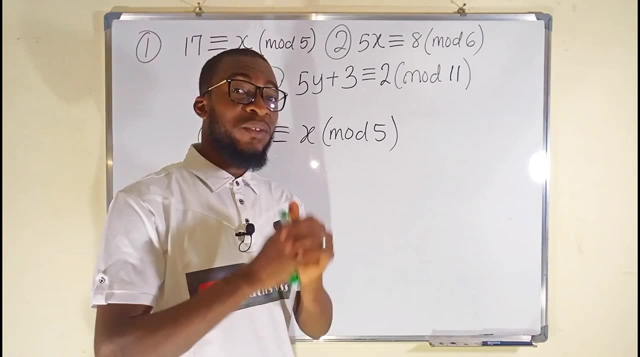 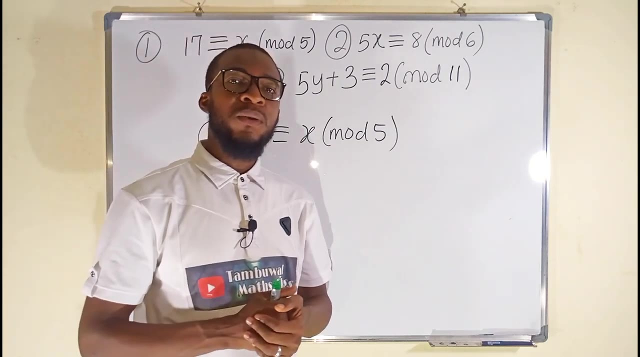 now talking about bundles of 5: 1, 2, 3, 4, 5. you recount all over again: 1, 2, 3. all the countings will be based on 5, which is a complete bundle, so 17. how many bundles of 5 are there? in 17 we have three groups. well, let me say we have. 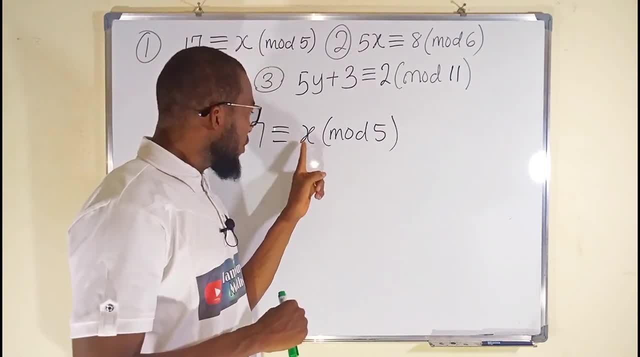 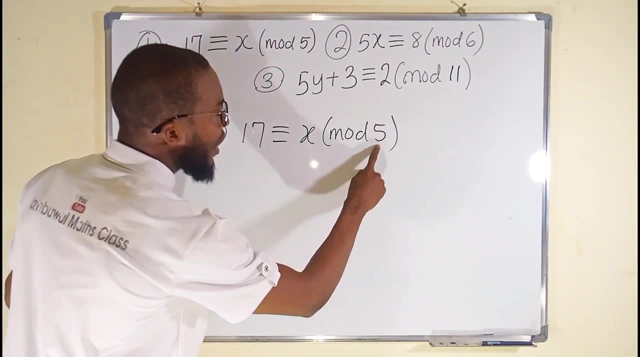 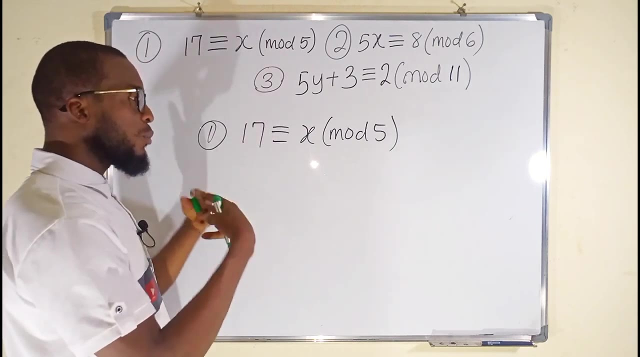 three bundles with a remainder of 2. so this number right here is just our remainder. what does this mean? it means that if we should divide 17 by 5, what is going to be the remainder, and that remainder is going to be our solution. so this time around you can even do it practically. you say 5 plus 5 plus 5, since 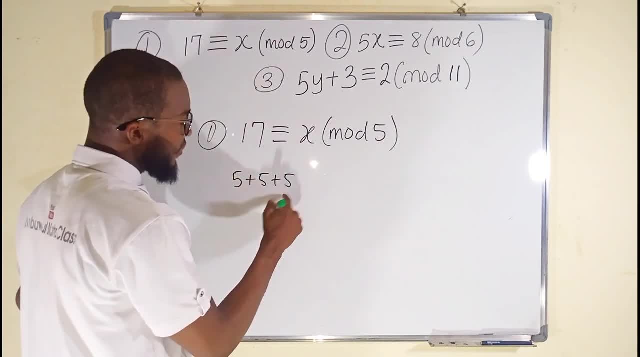 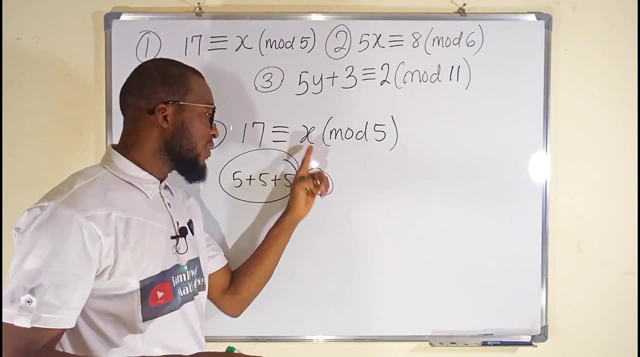 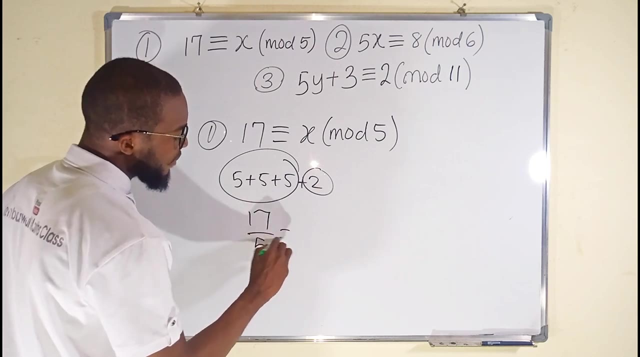 we are counting in bundles of 5, this is 15. then plus 2. can you see this is complete bundle, where we have a remainder of 2 and therefore this X is equivalent to 2. another way you can do that is to say that this 17 divided by 5 is equal to 30, which remainder of 2, and 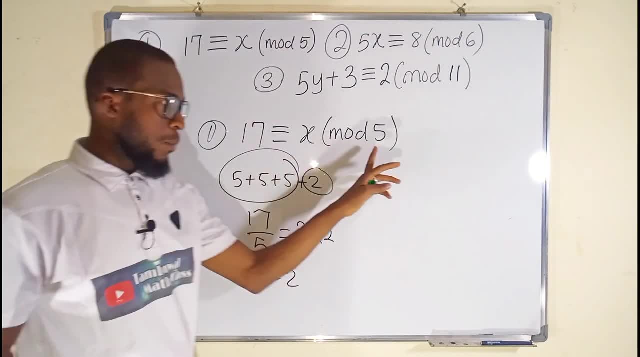 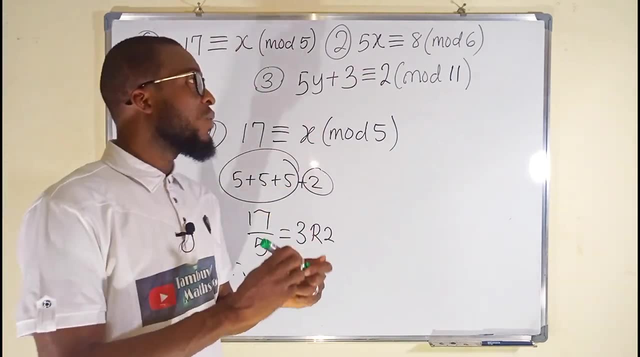 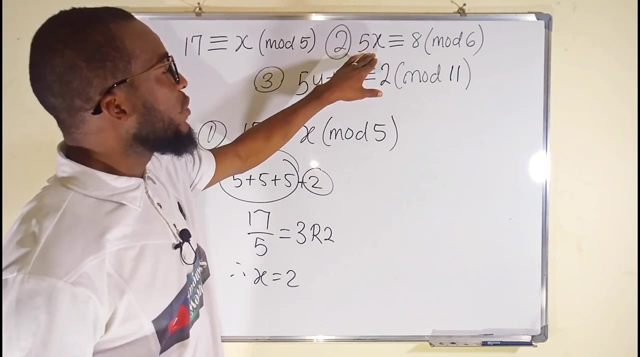 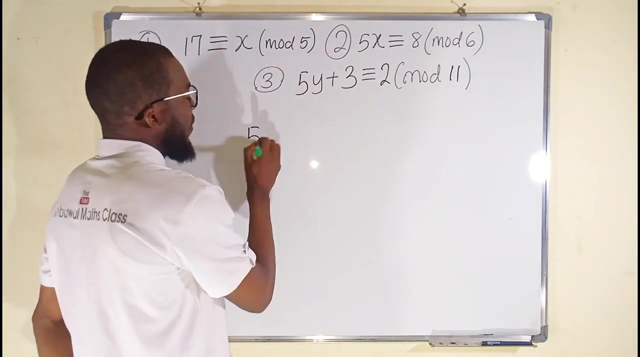 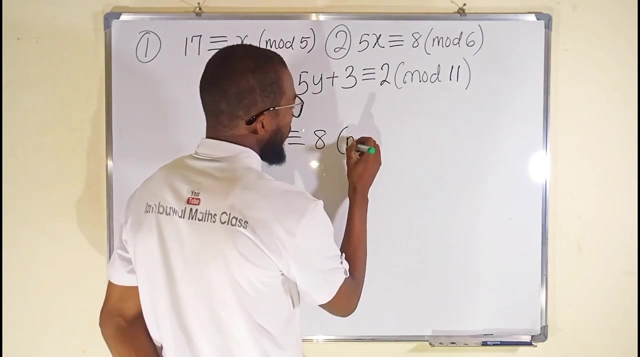 therefore, X is equal to 2, but only in mod 5. okay, second question: we have that 5x is equivalent to 8. this time around, this 8 is our remainder. so how many bundles of 6 are there in such a way that the remainder will be 8? so we have that 5, x is equivalent to it, but in 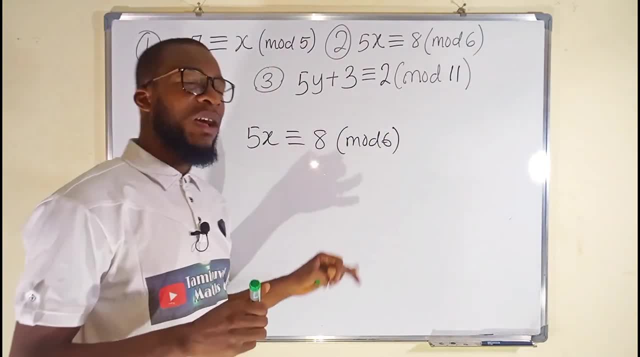 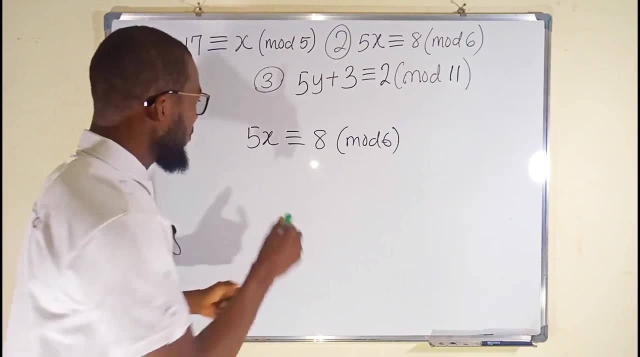 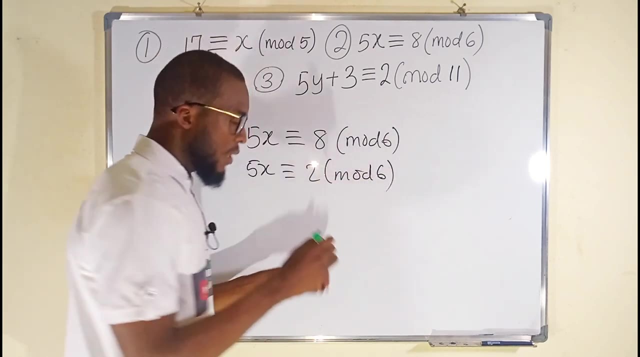 mod six. remember I told you that the highest we can have is 1, less than the mod is 10, but this time around we have eight. we this to two, it's the same thing. so we have five x equivalent to two in mod mod six, because if you divide this by six, you're going to get one with a remainder of two. so this: 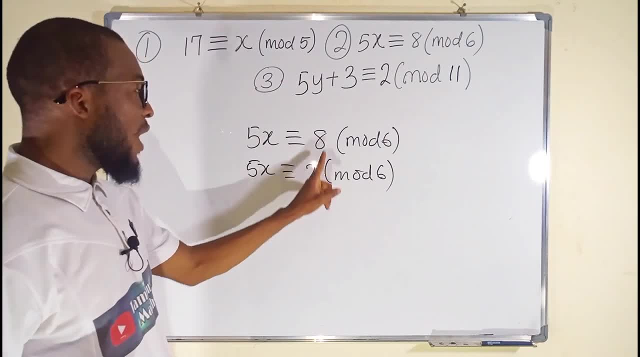 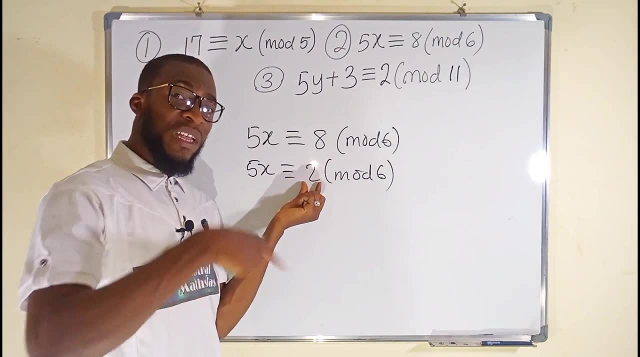 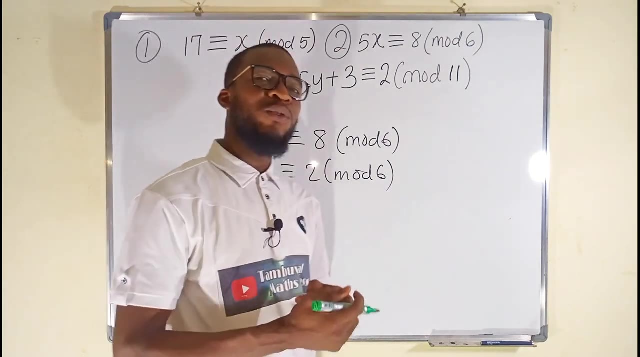 and this means the same thing, but it doesn't matter. we we're going to arrive at this eight again, because we are going to add multiple of six to this number until it gets a number that is divisible by five, because we cannot just say divide both sides by two, the way we normally do. 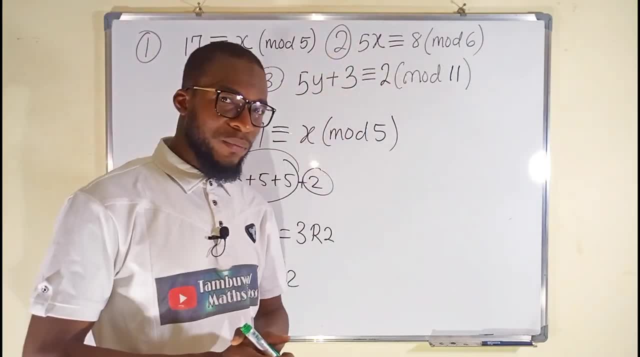 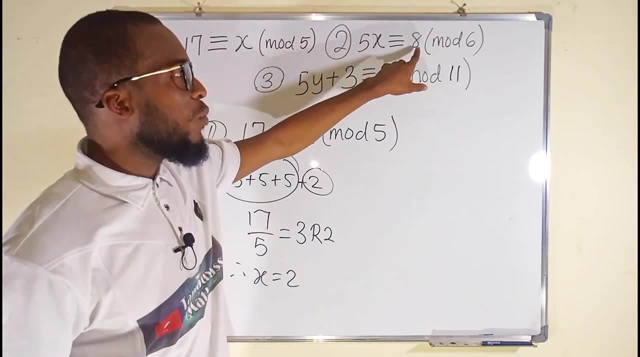 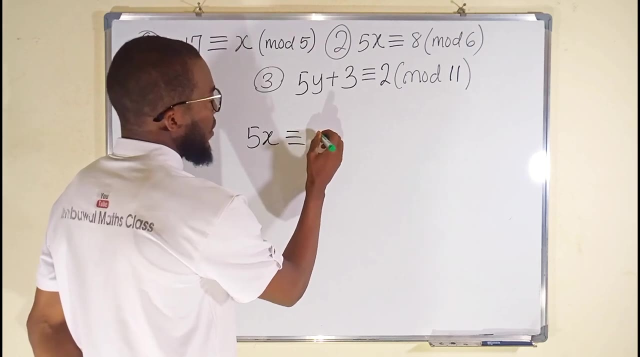 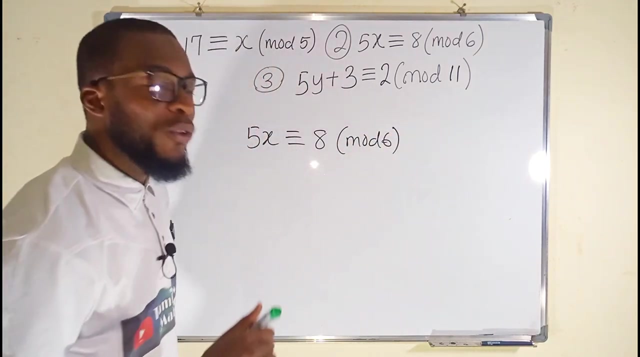 8. this time around, this 8 is our remainder. so How many bundles of 6 are there in such a way that the remainder will be 8?? So we have that 5x is equivalent to 8, but in mod 6. Remember I told you that the highest we can have is 1 less than the mod is there. but this time around we have 8. 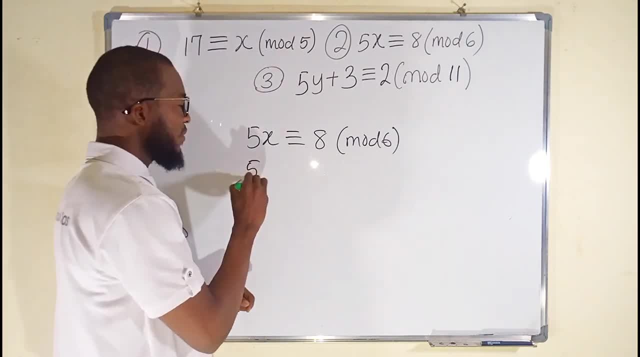 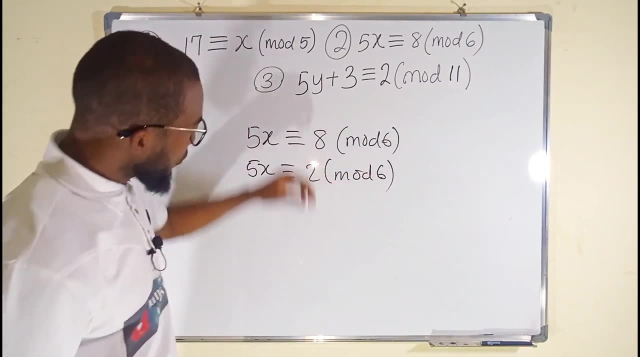 We can reduce this to 2, it's the same thing. So we have 5x equivalent to 2 in mod mod 6, because If you divide this by 6, you are going to get 1 with a remainder of 2. so this and this means the same thing. 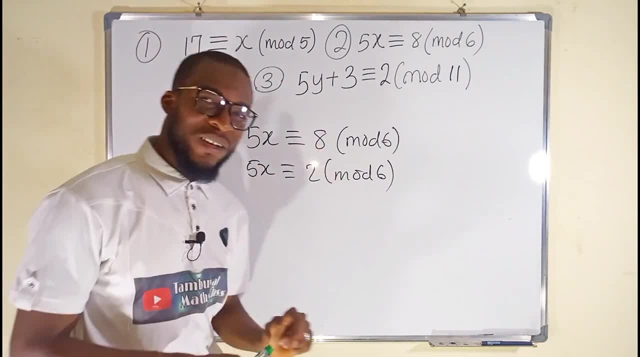 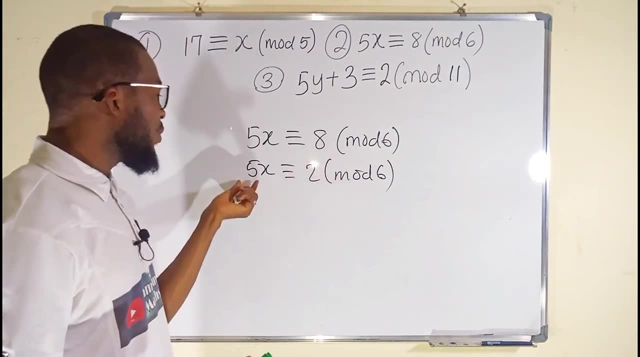 But it doesn't matter. we are going to arrive at this 8 again, Because we are going to add multiple of 6 to this number until it gets a number that is divisible by 5, Because we cannot just say divide both sides by 2 the way we normally do in linear. 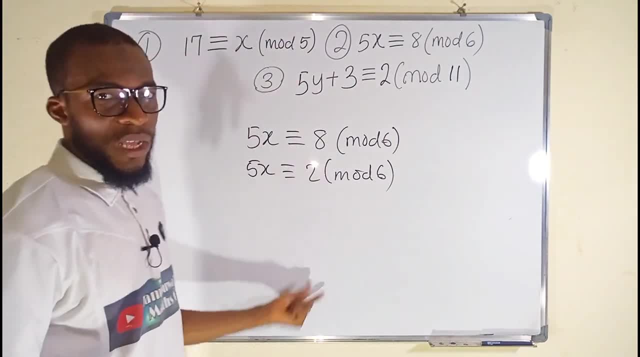 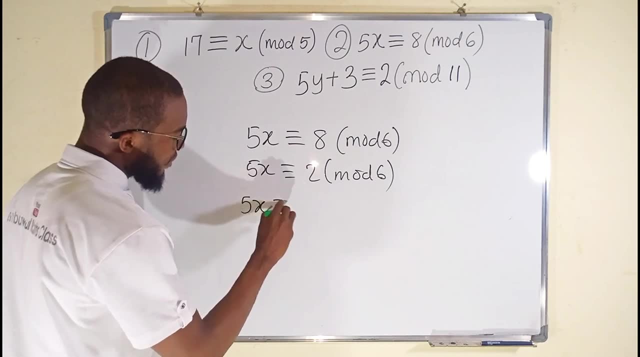 Algebra, because it is going to give us a fraction here, but we are concerned with positive integers. So this is equivalent to 5x, Which is equivalent to 6 plus 2, which is 8. you see, we have come back to what we have earlier. 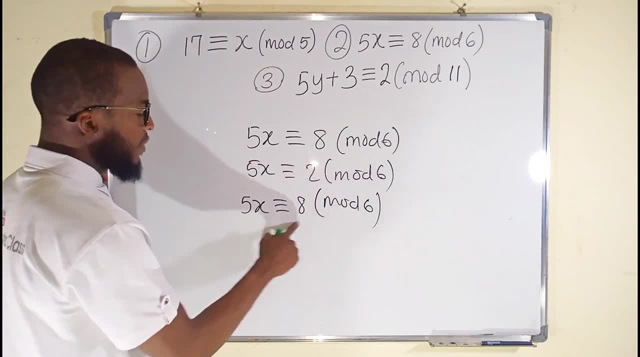 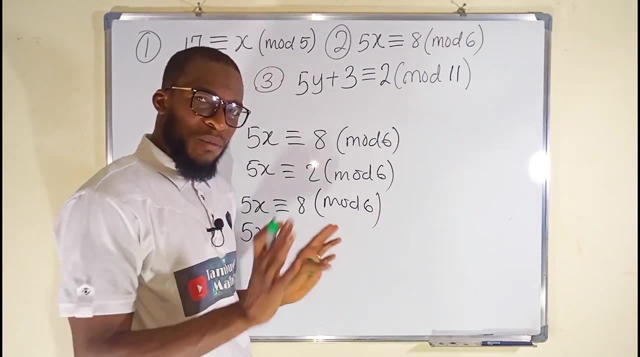 mod 6, but again, this is not divisible by this, so we carry out the Add again is just like at a 0. Complete bundle is the same thing as 0. This is equivalent to 8 plus 6 again. This is 14. 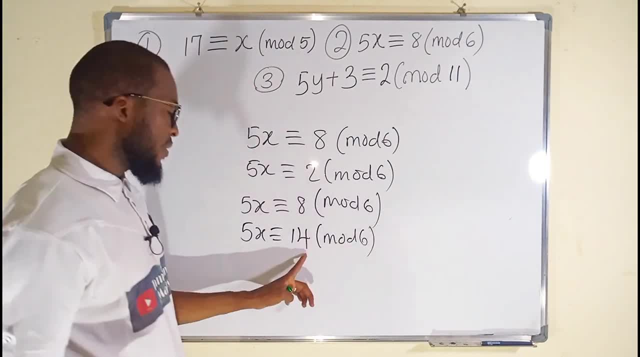 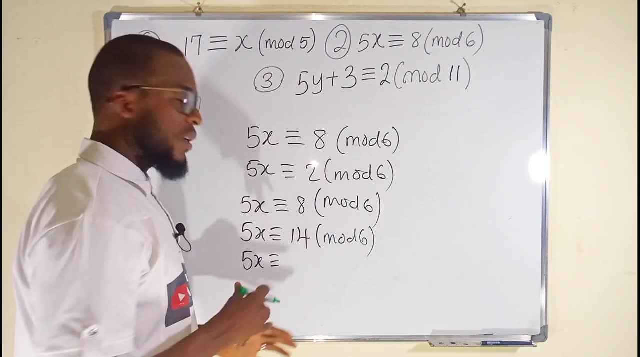 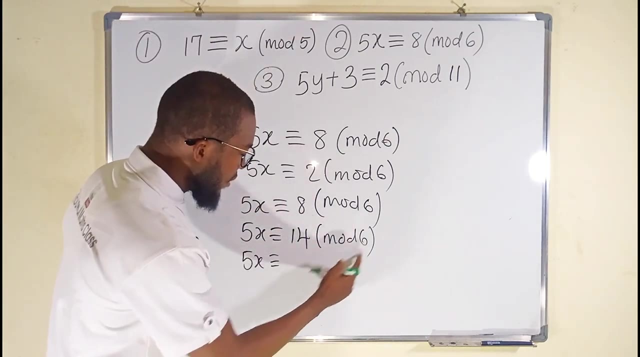 mod 6. Again, this is not divisible by this. We continue adding 5x. I want to do it practically. I know I can just add it directly. I can add that number directly to this so that it will be divisible by 5, But I just want to show you the steps. this plus this is now going to give us 20. 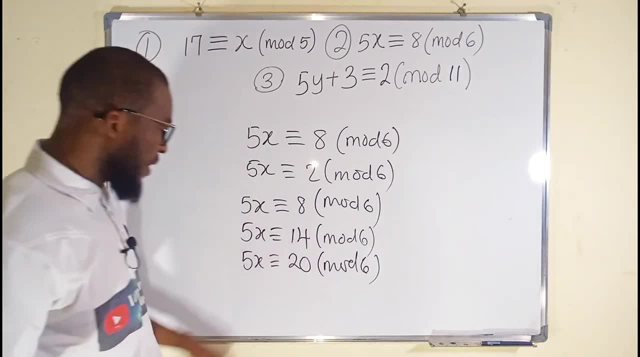 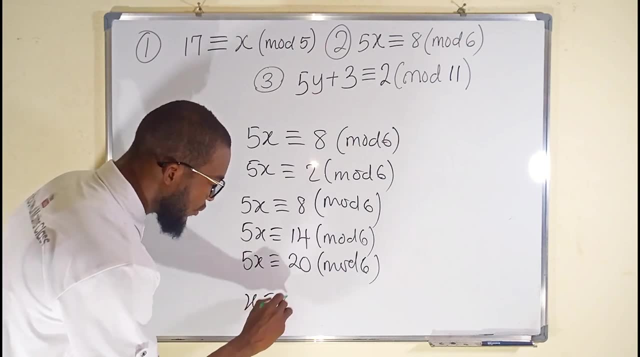 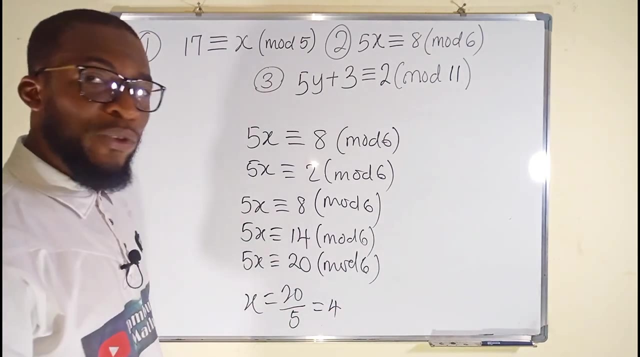 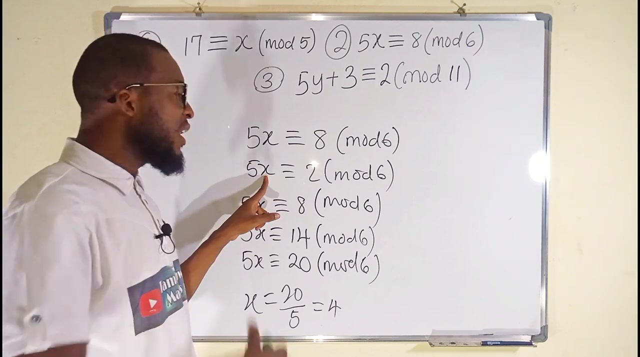 mod 6. But now that 20 is divisible by 5, we can conclude this: this X is equal to 20 divided by 5, which is equal to 4. therefore, the value of X is equal to 4, and we can test it here 5 times. 4 is 20, and how many groups of 6 are present in 20?? 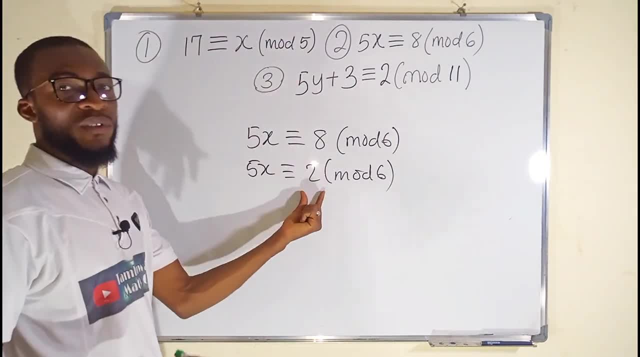 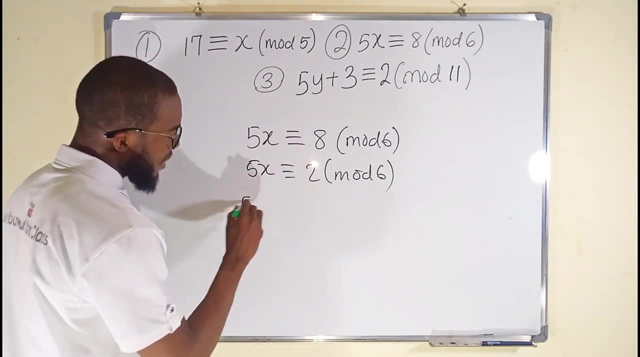 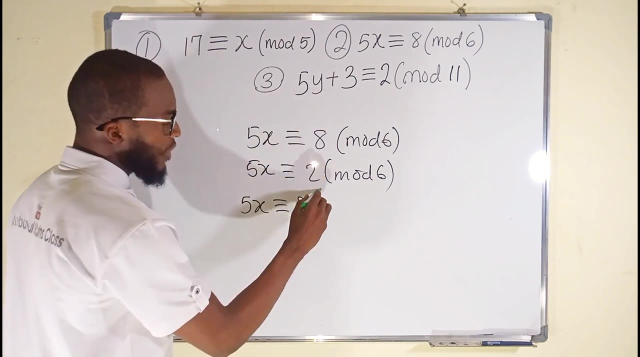 in linear algebra, because it is going to give us a fraction here, but we are concerned with positive integers. so this is equivalent to five, x, which is equivalent to six plus two, which is eight. you see, we have come back to what we have earlier, mod six. but again, this is not divisible. 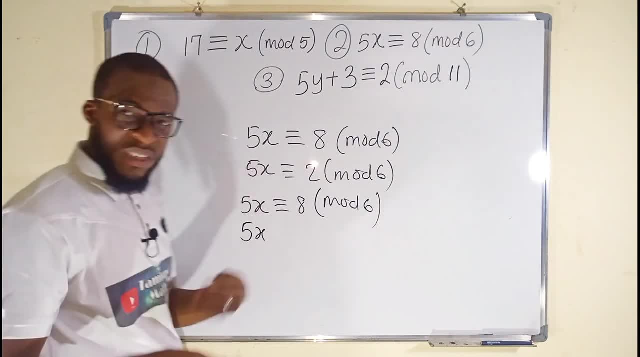 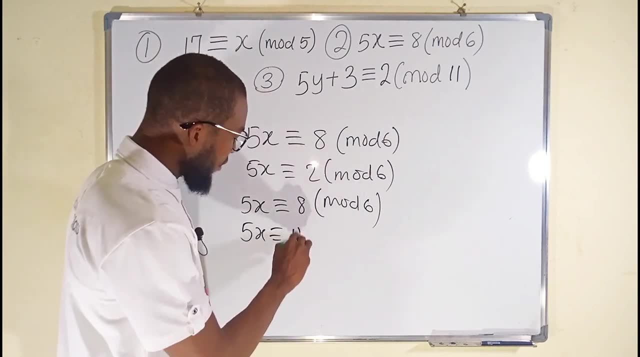 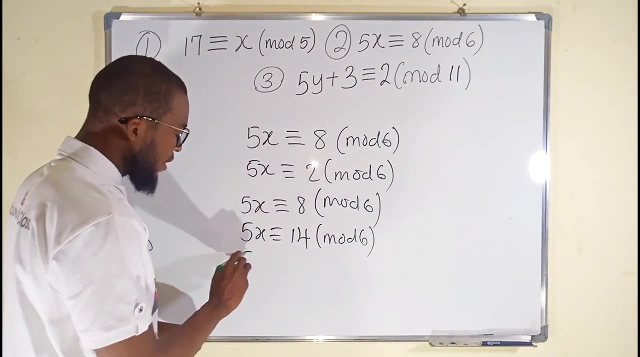 by this so we can add again. it's just like at a zero complete bundle is the same thing as zero. this is equivalent to eight plus six. again. this is fourteen mod six. again. this is not divisible. by this. we continue adding five x. i want to do it practically. 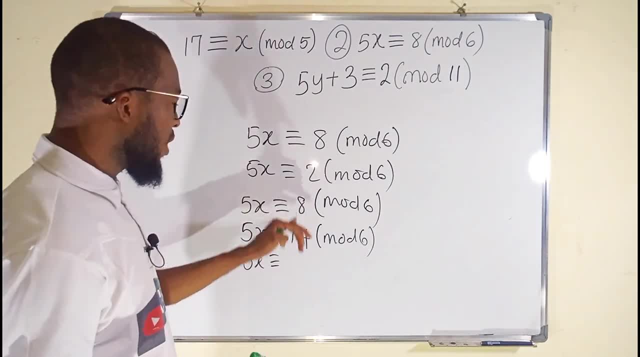 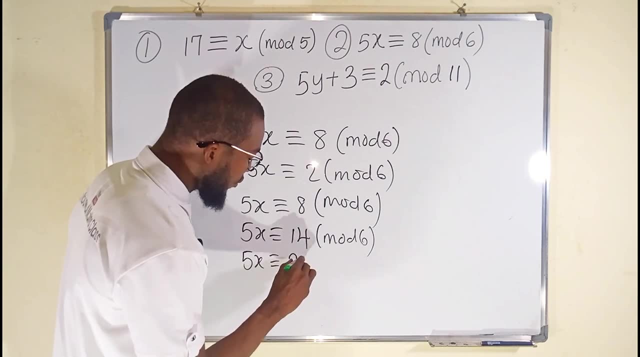 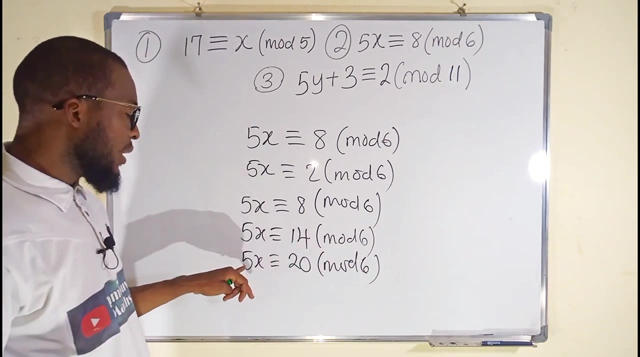 i know i can just add it directly. i can add that number directly to this so that it will be divisible by five. but i just want to show you the steps. this plus this is now going to give us 20 mod six. but now that 20 is divisible by five, we can conclude that this x. 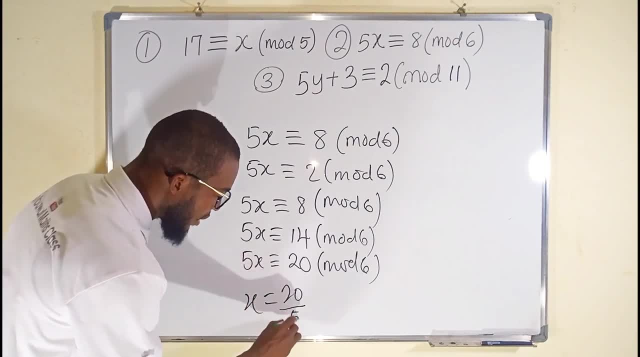 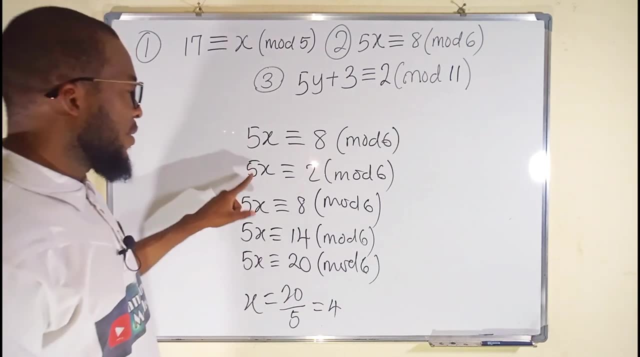 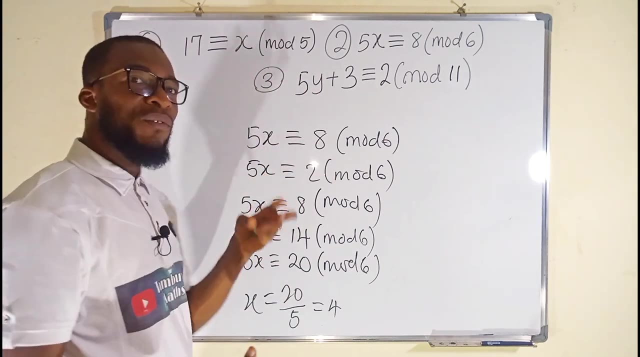 is equal to 20 divided by 5, which is equal to 4.. therefore, the value of x is equal to 4.. and we can test it here: uh, 5 times 4 is 20.. and how many groups of 6 are present in 20? we have three groups. 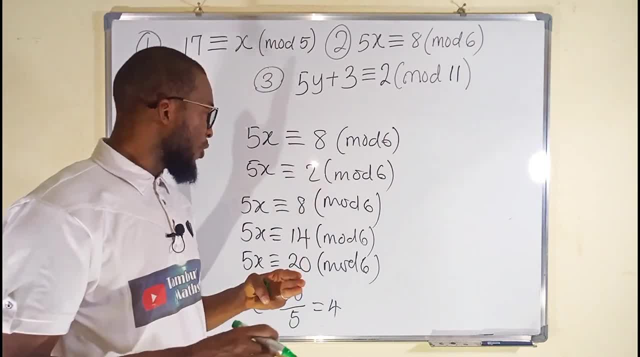 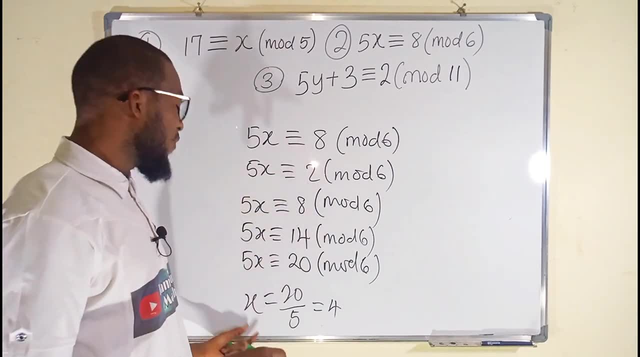 6 plus 6, 12 plus 12 is 18, but 18 is 2 less than 20, so we have a remainder of 2, which satisfy the equation. therefore, the value of x is equal to 4.. let us take the last one. 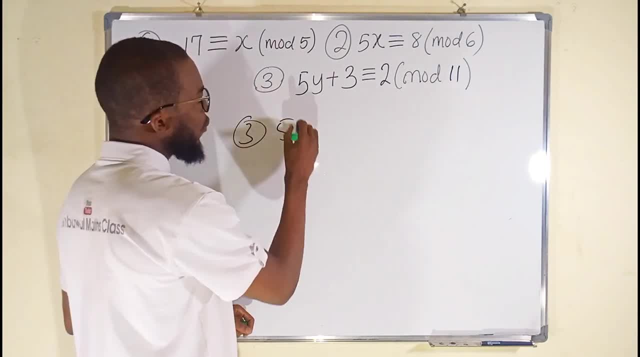 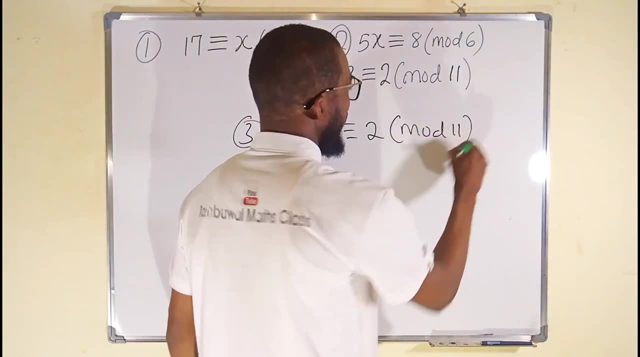 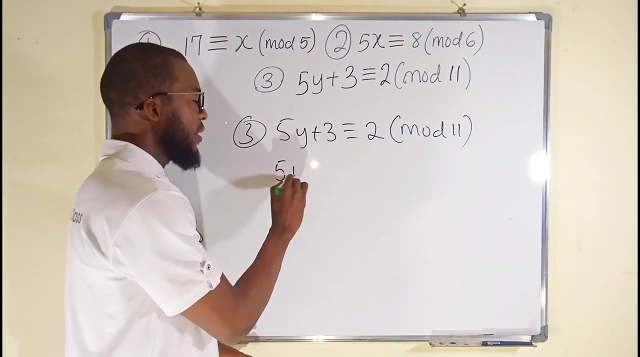 the last problem. we have that 5y plus 3 is equivalent to 2 but a mod 11.. let us first of all take this time. here we have that 5x, or let me say 5y, is equivalent to negative 1, because 2 minus 3 is negative 1. 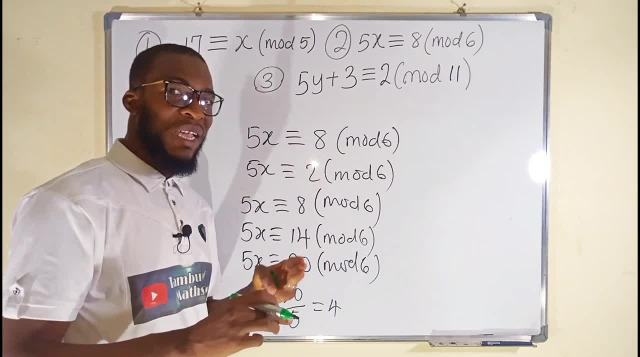 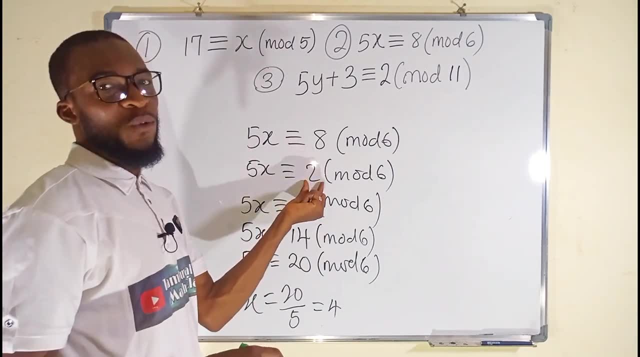 We have three groups, because 6 plus 6, 12 plus 12 is 18, But 18 is 2 less than 20.. So we have a remainder of 2 which satisfy the equation. Therefore, the value of X is equal to 4.. Let us take the last one. 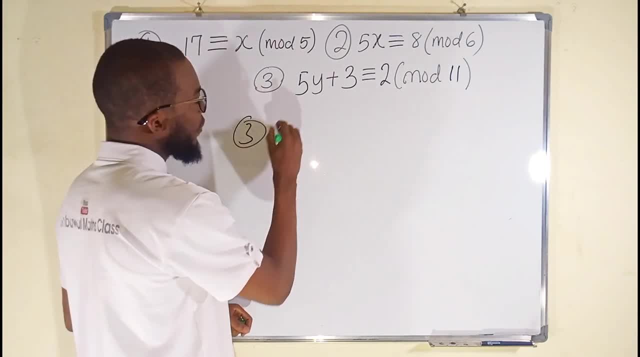 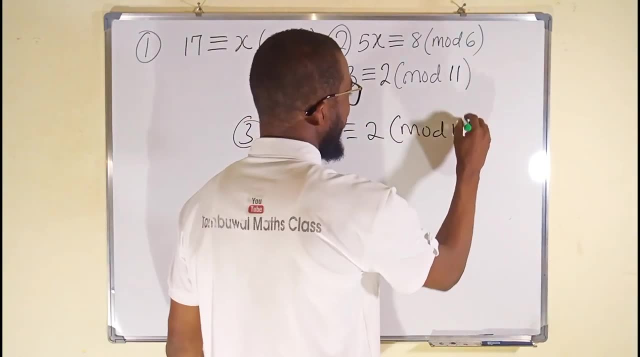 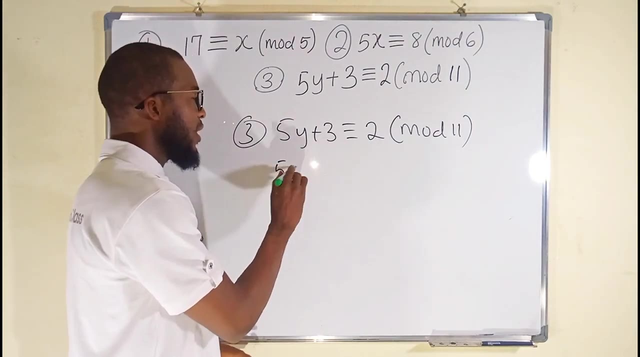 the last problem. We have that 5y plus 3 is equivalent to 2 but a mod 11. Let us first of all take this time. here We have that 5x- Let me say 5y- Is equivalent to negative 1, because 2 minus 3. 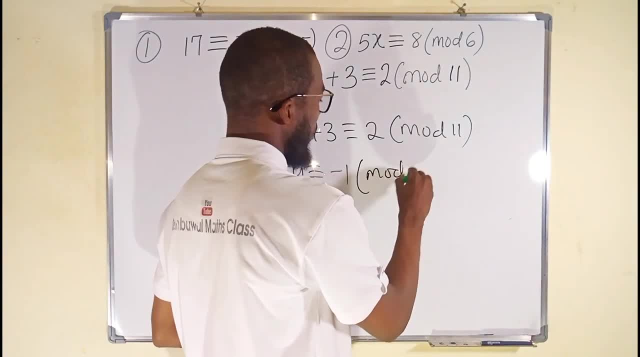 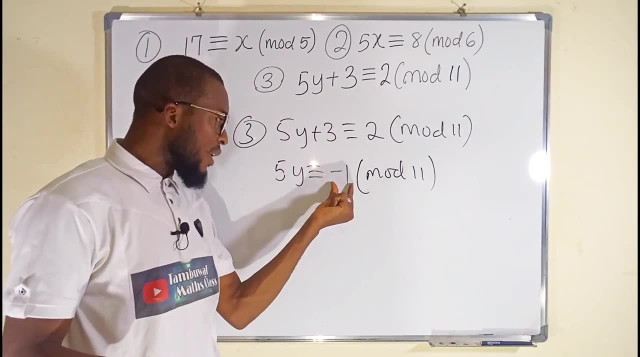 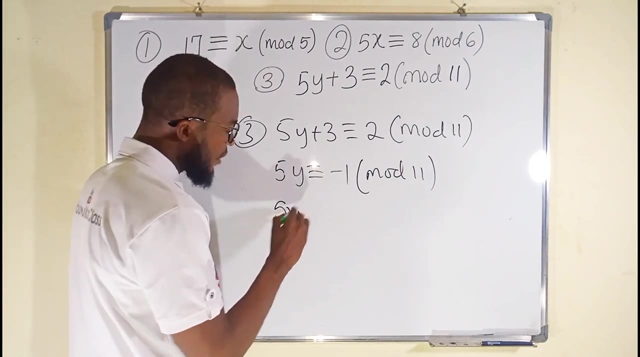 Is negative 1 and mod 11, We're going to repeat the same process. We are going to add multiple of 11 to this number until it gets to a certain value Which is divisible by 5? So this 5y is also equivalent to 11. 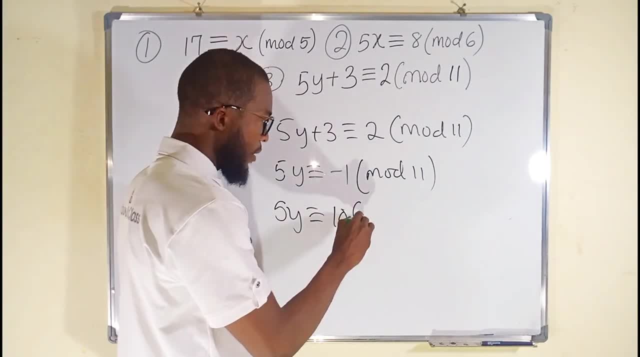 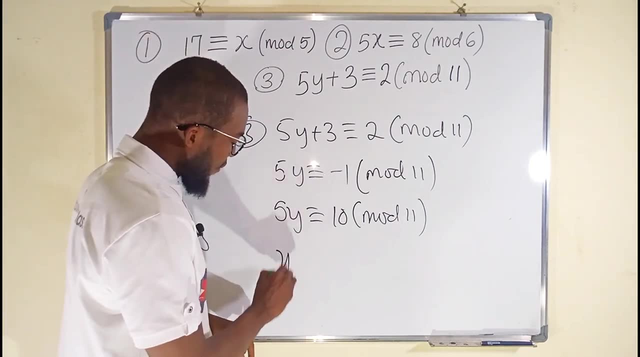 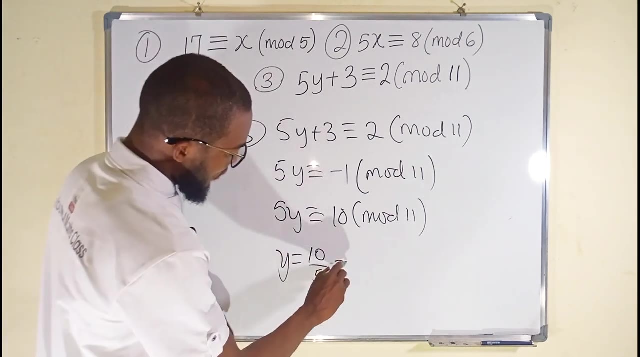 Plus negative 1 is going to give us 10 In mod 11. let's stop here, because 10 is divisible by 5. Therefore, we can say that 5 is equal to 10 divided by 5 and this is equal to 2. it means that the value of Y is equal to 2.. Let's see whether this is true. 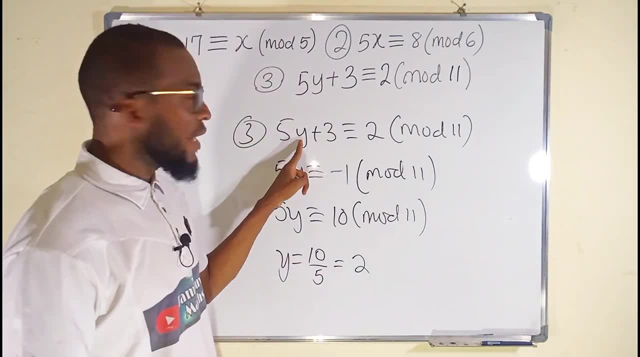 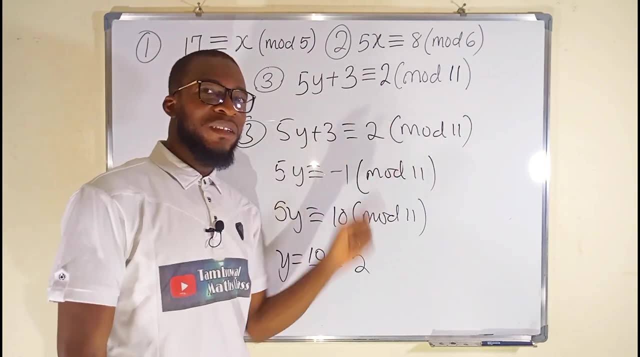 So if Y is 2, we have that 5 times 2 is 10, and 10 Plus 3 is 13. How many groups of 11 are there in 13?? We have only one, 11, and from 11,, 12,, 13. 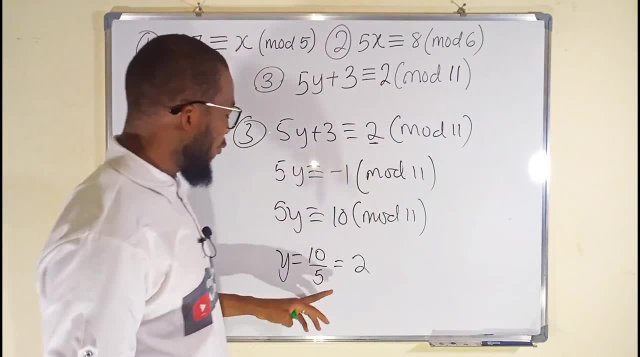 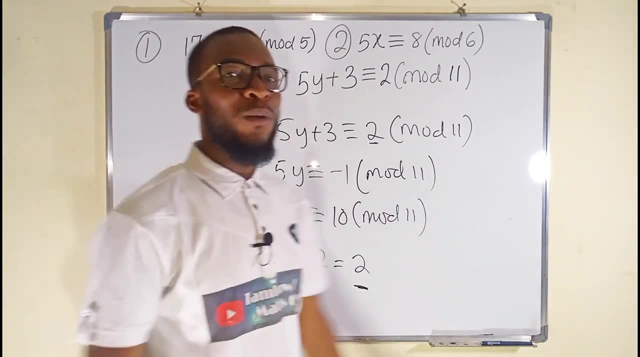 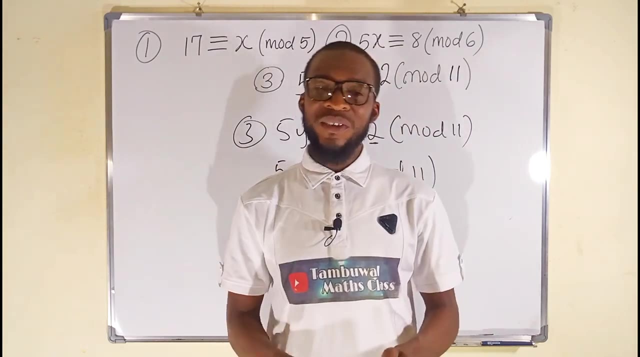 We have 2 remainder, which is this, therefore: Y equal to 2 satisfy this equation, and hence we say that Y is equal to 2 is our Valid solution, and this is all I have for you today. Thank you for watching. Do share to your learning colleagues and don't forget to subscribe to my youtube channel for more exciting videos. Bye, Bye. You.